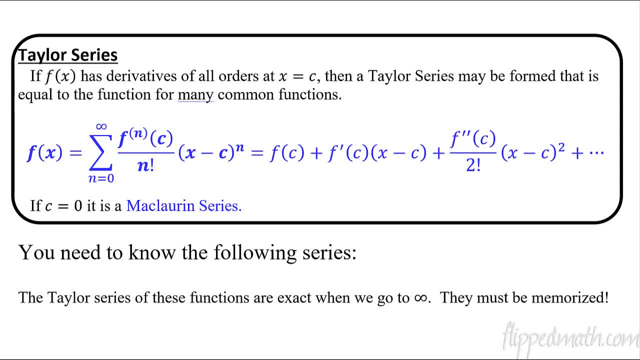 series is similar to a polynomial series. We've done this before, so if you'll notice, this is hopefully you're starting to write this down. You've got this big long thing here and it is very similar to what we've done before. You have f of. 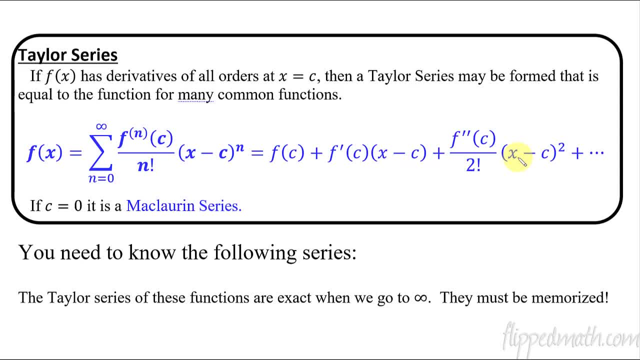 C plus f, prime of C times X minus C, and so forth. It follows the same pattern as a Taylor polynomial, What the series does. if, when you add all of these terms together, that series actually equals the function for many common functions that we work with That summation, the series here actually is the function which is: 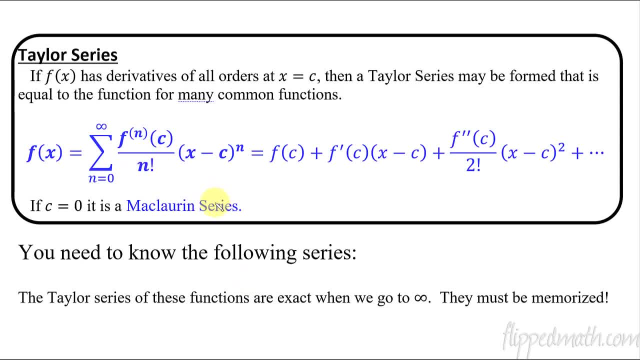 kind of cool. Now, typically, we're gonna work with a Maclaurin series, So you're just gonna have the centered at C equals zero and you won't have to worry about this minus C part in all these, and we'll just say the C is a zero For most of. 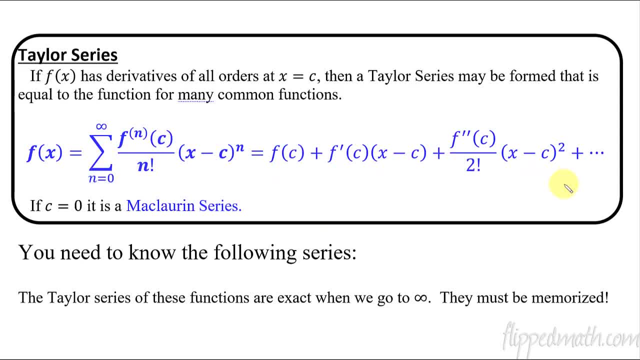 stuff that we'll be doing. it'll be like that, But I wanted to put the Taylor series part in the middle so that you can see the difference between the two Here, just so you knew that one and then the Maclaurin is easier. So what we're? 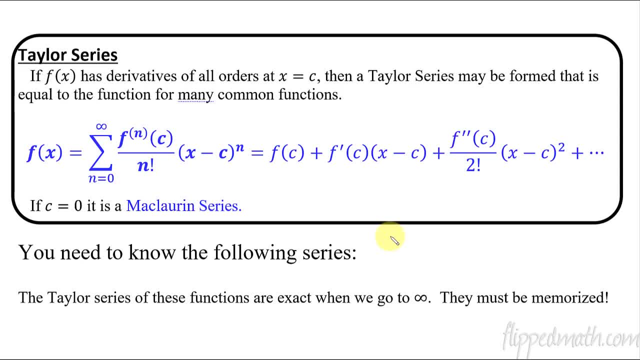 gonna do today is you're gonna learn the following series, These four. We're gonna get these figured out. What is the? what is the Taylor series for these four, Specifically the Maclaurin series. actually, We're gonna do the Maclaurin. 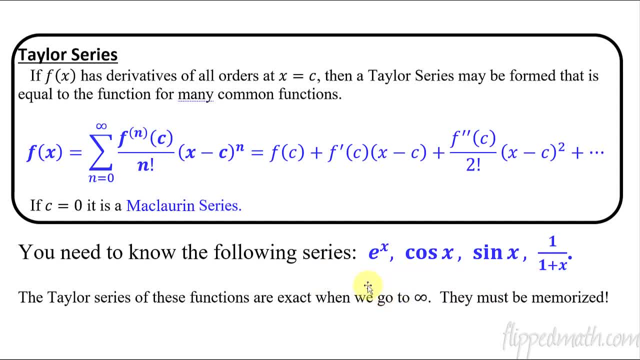 series for these four things. and then you got to get it memorized Because if we know these four, you're gonna be able to work with them and manipulate the Taylor series based on what the Taylor series is of these. Okay, that was confusing. I just talked in circles, You'll see. 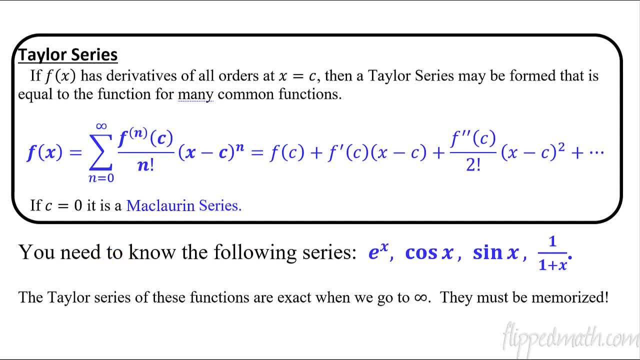 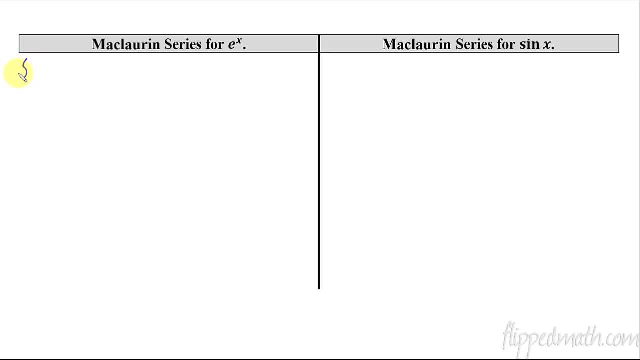 what I mean here when I get to the examples. So get this written down. if you don't, and let's get into figuring out what is the Maclaurin series for this first one: E to the X. So again, if you, if you don't have it memorized, you could do. 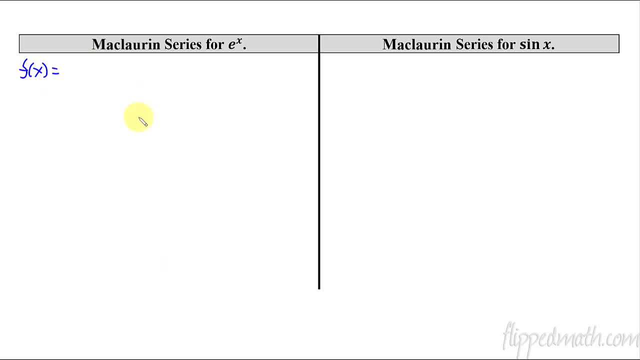 this the long way, which I'm gonna do for this first one, But that just takes a while, so it's a lot better if you're gonna be able to memorize these. So let me show you this. So f of X is going to be if we centered at zero. it's going to 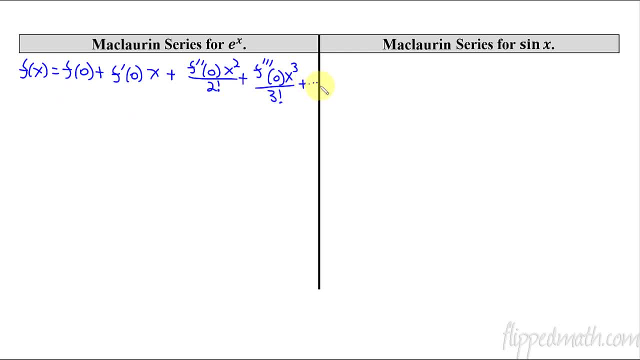 be this thing, and then it continues on. See, I have this plus dot dot dot, So hopefully this is familiar. We've done this before. So here's how we set up the Taylor series. In this case it's a Maclaurin series because it's centered at 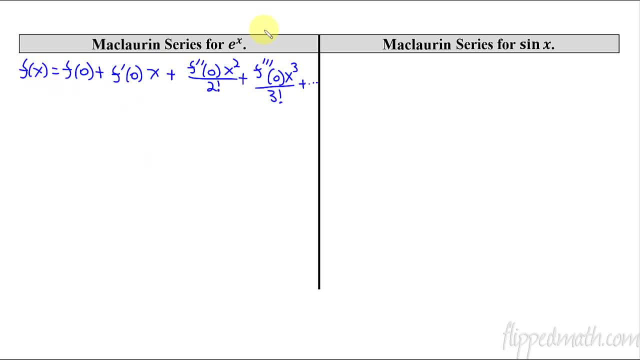 X equals C equals zero. Now the function that we're working with is E to the X. So let's go ahead and write out: E to the X is going to equal. Now the, the f prime. on all of these f prime, second derivative, third derivative, that's all gonna be E. 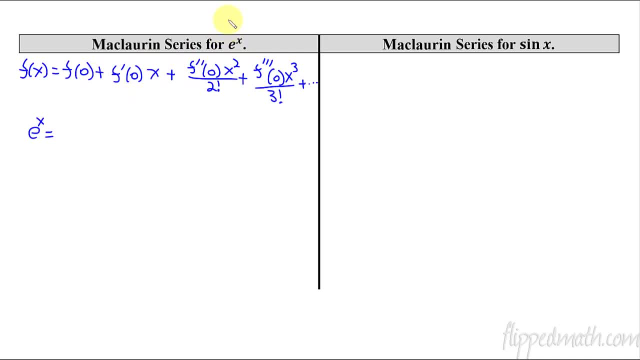 to the X. So those will all be the same answer. and we know that E to the zero. well, that equals one. So every single one of these- f prime of zero, f, double prime of zero, those are all one. So that makes this really easy. So what happens here? 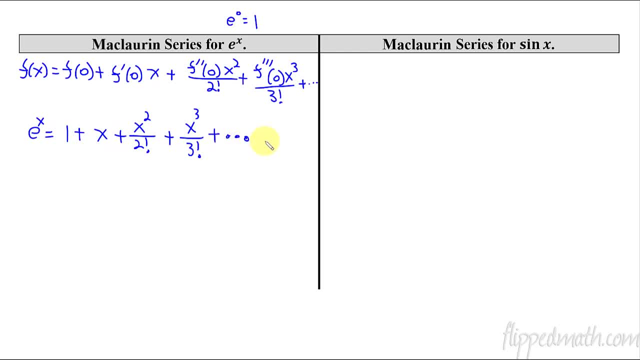 this is going to be this thing here, and it continues on and on and on until you get to now- we could write a pattern of this- is just until we get to X, to the nth power over n factorial, And what we're doing is we're going to end up. 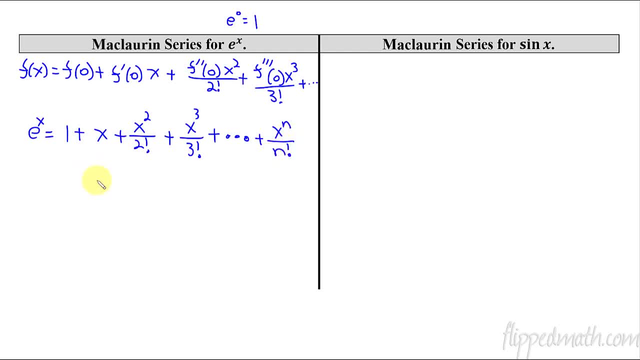 having. if we want to have a summation notation of this, we're going to just say: this is the sum as n starts at zero and goes off to infinity of this nth term. So we say of X to the n over n factorial. This is what you are going to memorize, this line and this line, these two things. 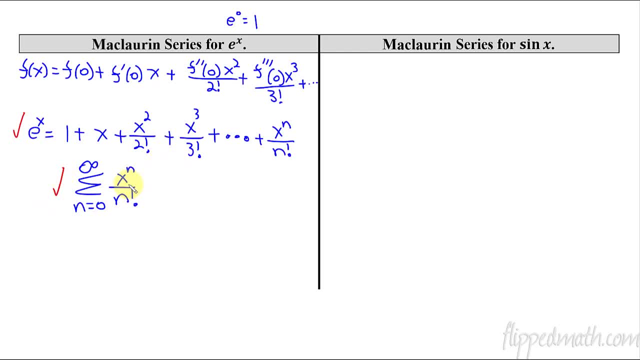 you want to have that memorized Now. I've got a chart here later in the notes where we're gonna organize all of this so you can have it all in one place where you look for your notes. And then, if we did a ratio test and we, using the 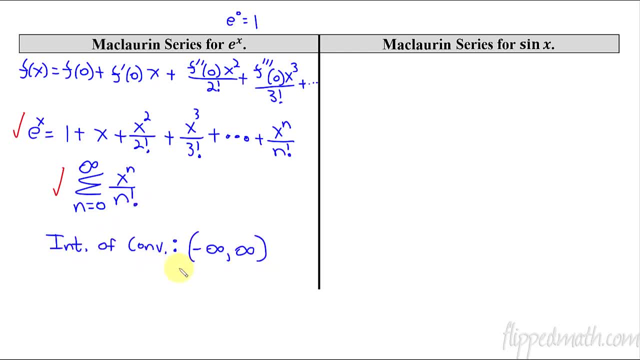 ratio test, we could figure out the interval of convergence, and that interval of convergence would be from negative infinity to infinity for this thing. Alright, so that is the Maclaurin series for E to the X, and we memorize that because we're gonna use it to figure out other things like the. 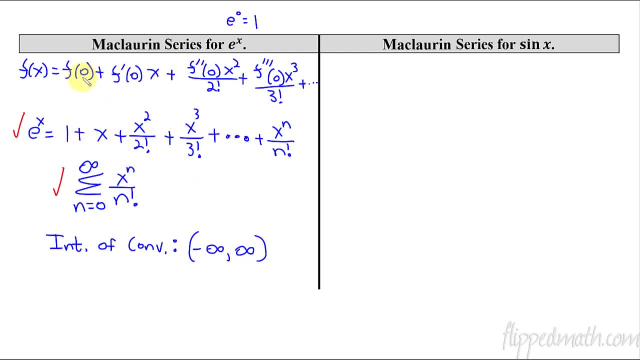 integral of infinity. So if you have other problems and if you haven't memorized, then it's really easy. If you have to do this the long hand every single time, it's gonna take you a while. Okay, so I'll come back to this and talk. 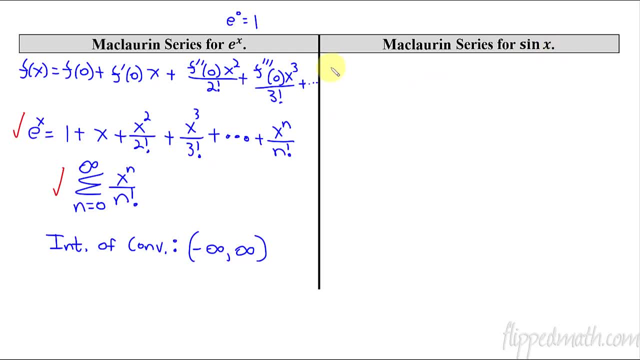 about this a little bit. Let's now figure out. what about sine X? What is that one gonna be? So I'm gonna write out again. oh, wait, to do this one, we need to write a list real quick. What is F equal? F is sine. The derivative of F is cosine. Second, 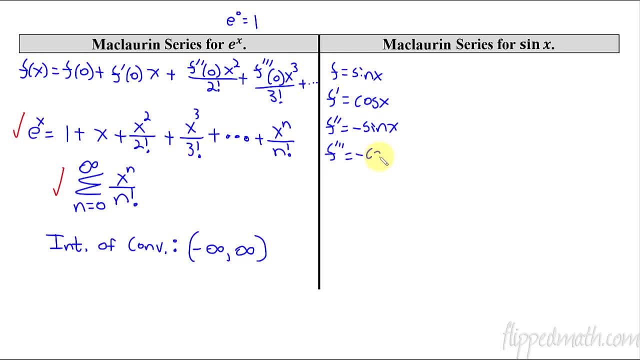 derivative of F is negative sine. Third derivative: negative cosine. And then if we took the derivative of that and got the fourth derivative, we'd be back to sine, And so it repeats this, this order, over and over again. Alright, so now, since we're doing a Maclaurin, let's figure out what's F of zero and F prime. 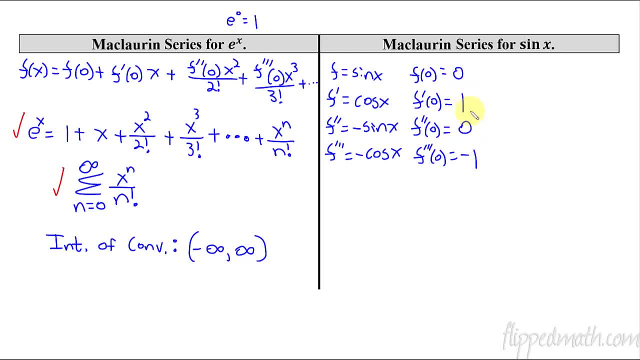 of zero and so forth, And it will get this pattern: 0 1 0 negative. 1 0 1 0 negative 1.. That's the pattern over and over again. We're gonna use this line right here and use the same thing to plug in the stuff that we need to come. 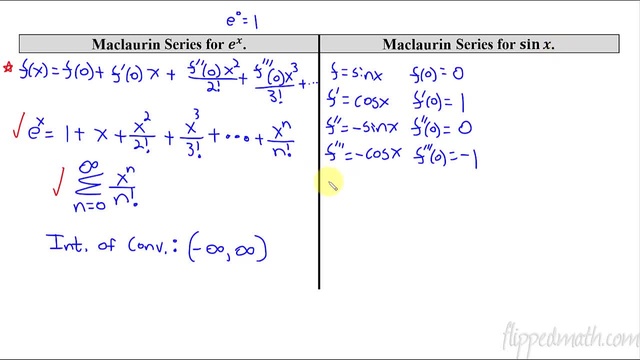 up with the Maclaurin series for sine X. So we'll write out that sine X is sine X. So we'll write out that sine X is sine X. So we'll write out that sine X is sine X. And then we start plugging stuff in. So let me has that just. 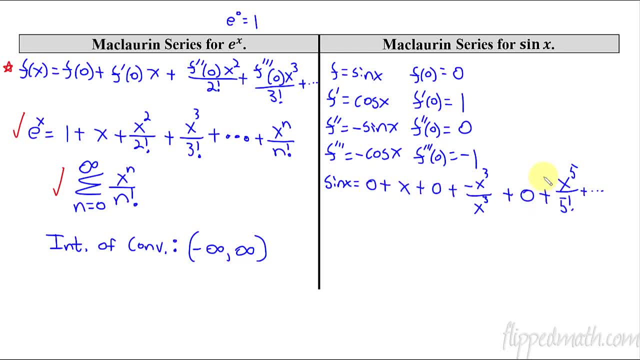 appear here. So you get this thing where every other term is gonna be end up being a 0, because every one of these, every other one of those, is 0.. Oh wait, sorry, some of you caught that. I made an error. Let me fix that right. 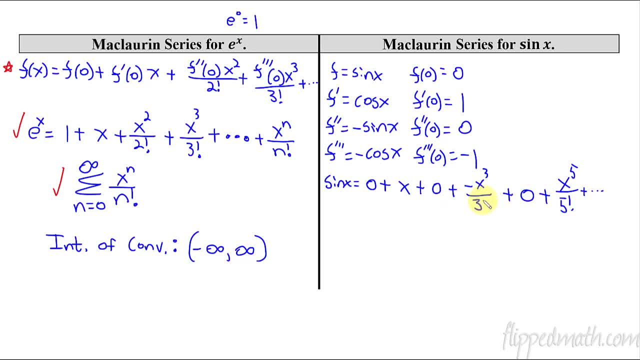 there I put hex cubed because I'm not paying attention what I'm doing- And it should be three factorial. okay there. Now let's go on and clean this up a bit and write down the next line. Alright, so now we have this pattern. Notice how the exponents are all odds. 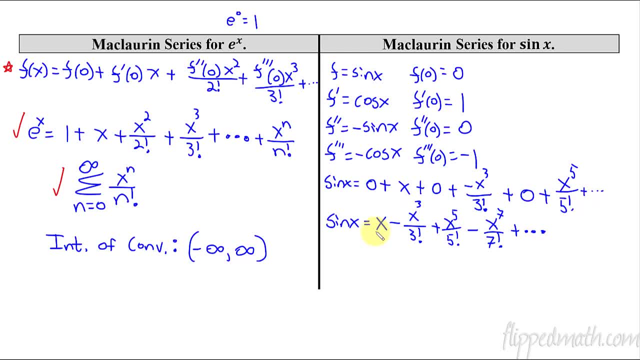 1, 3, 5, seven, nine, eleven, so forth, and so then the denominators would also be the odds: one factorial, three factorial, five factorial. okay, so that's gonna help you with the memorization. the sign is gonna be all the odds, and when we get to this, 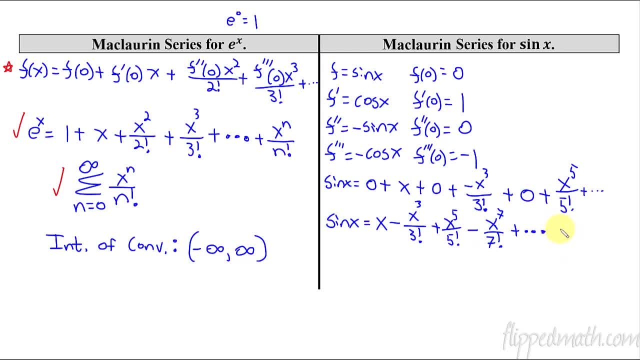 last part- this is the part that's gonna be a little bit harder to memorize- that very last term, the nth term, it's this crazy thing. so it's alternating. every other term is positive and negative, positive, negative, and then we're going to be starting at 2n and then plus 1 to get this 1, 3, 5, 7, and then it's the same. 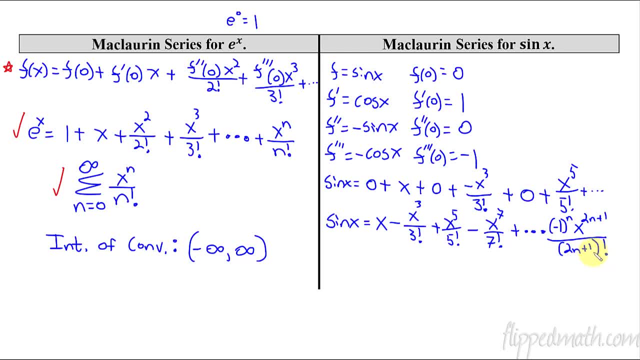 thing 1, 3, 5, 7 will be 2n plus 1 on bottom factorial. alright, then our last step is we: we write out what is the summation. so the summation notation is just gonna go from 0 to infinity of this nth term. so then we just write that. 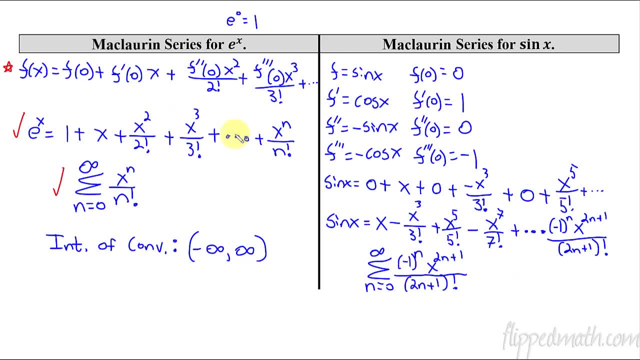 again, and there we go. so what are the things you're gonna be memorizing? you're gonna be memorizing this step right here, as well as this step. okay, so again we're. I'm gonna show you the chart. so here we go. let's put this all in the chart. 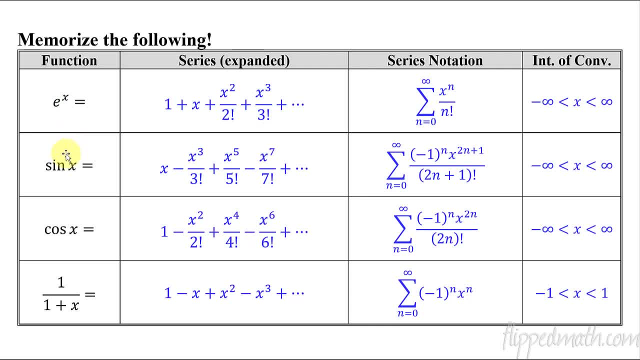 instead of us figuring out all of them. so I just showed you how we figure out e to the X and sine to the X. we're not gonna work out cosine and the 1 over 1 plus X. it's the same way you do it. so here is the chart that you're gonna fill out. so e to 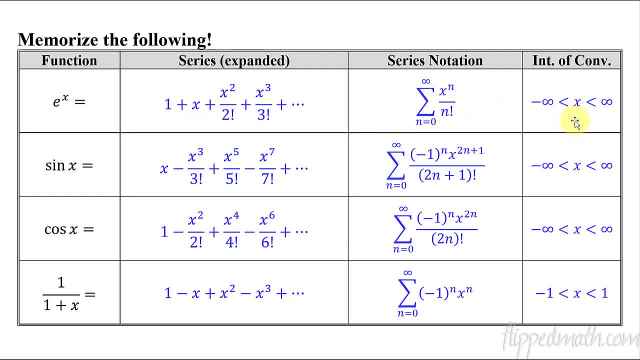 the X we did. and then here's the series notation interval of convergence. if we did the ratio test we could figure out all these interval of convergences. and then sine X, we just did. so what I would say is: notice that sine and cosine are very similar. the difference is what I try to remember. 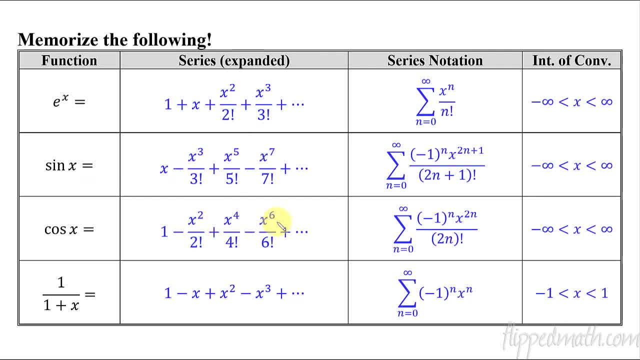 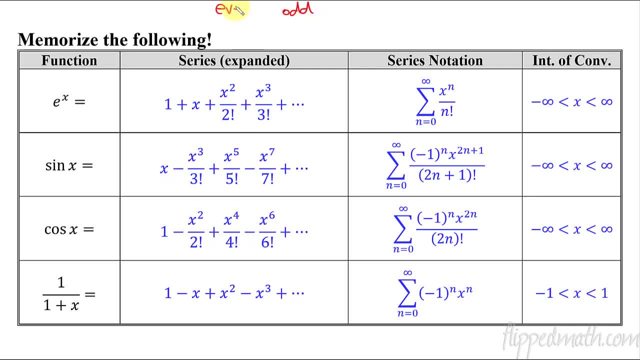 odd, and even it's alphabetical, and cosine and sine are also alphabetical, so it's cosine and sine. if you put them alphabetically then it helps you remember that cosine is with the evens, see two, four, six, ah. sine is with the odds alphabetically: one, three, five, seven. okay, kind of dumb but it works for me to help. 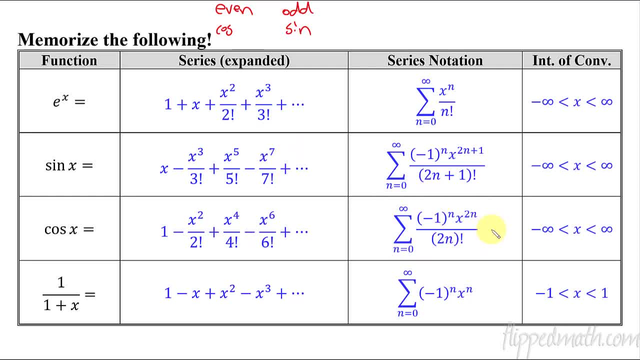 me remember these, and then this series notation you also want to have memorized. and then the one over one plus X. this is kind of a cool one. it alternates every other one and then it just increases X, so that's why it's negative. one to the end for alternating and X then. so pause, get, oh, but the. 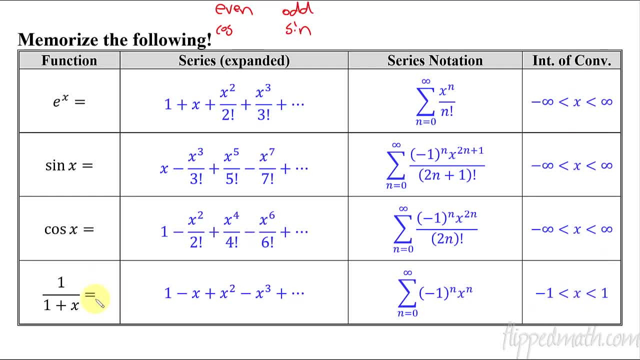 interval of convergence is only from negative one to one. so this one only works to tell us that. what this equals from this point. so pause the video, get this written down real quick. so let me remind you what this does. this tells us that if we take a series, this is equivalent to e to the X, this series, right here, this is. 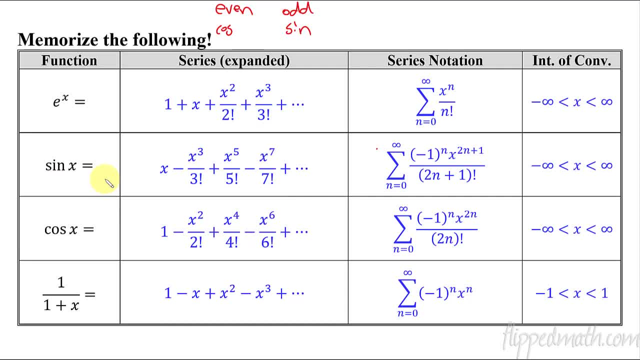 equivalent to sine of X. it doesn't work for every function, but it works for a lot of function, especially some of the common ones, and so these are the ones we're going to memorize that it works for, okay, so, before I jump into an example, let me show you one interesting thing, and that is that this one over one 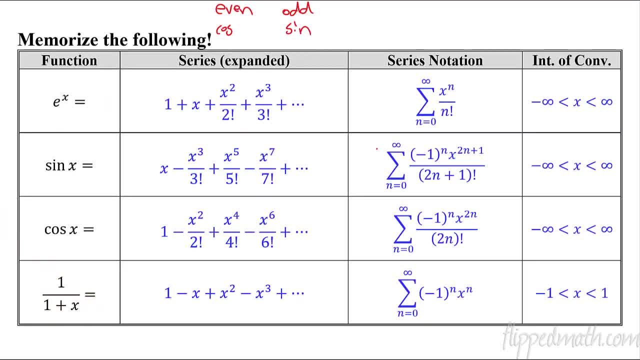 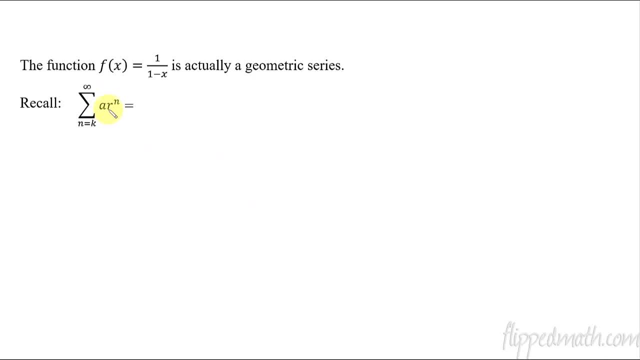 minus X, which is really close to this last one, one over one plus X. this is actually a geometric series which is kind of interesting. do you remember when we did this back in the second lesson of unit 10? we had geometric series and this formula would do exactly what we did in his test problem. now use what we did in. 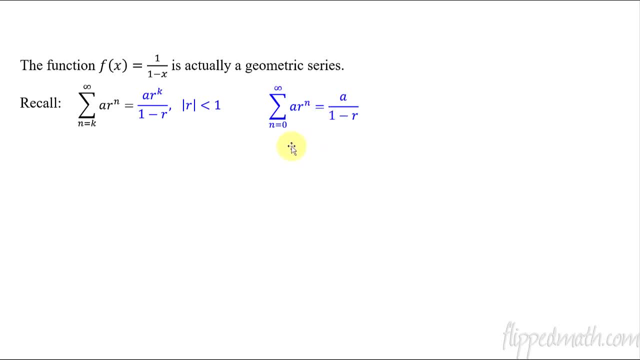 his example and write on: X is equal to Y. what we were looking for to would be a value. let me simplify this down a little. but that's interesting, really cool, because if you just take the circuit for that, much just doesn't materialize. well, you have a lot to do with what. 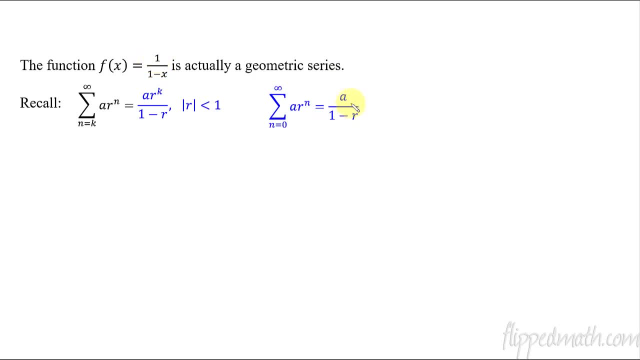 So what's the difference here? Well, we've got 1 and a instead. So what we're going to say is that a equals 1.. And instead of an x, we're going to- or instead of an r, we're going to say, x. 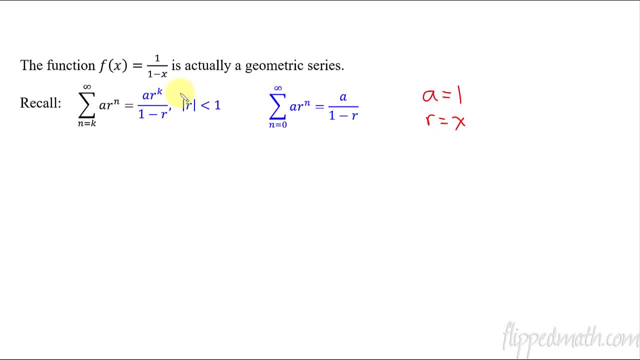 So r is going to equal x. So if we do that, then this can be represented. We can say that 1 over 1 minus x is the same thing as the summation of, and then we write this up. We're going to say n equals 0 to infinity. 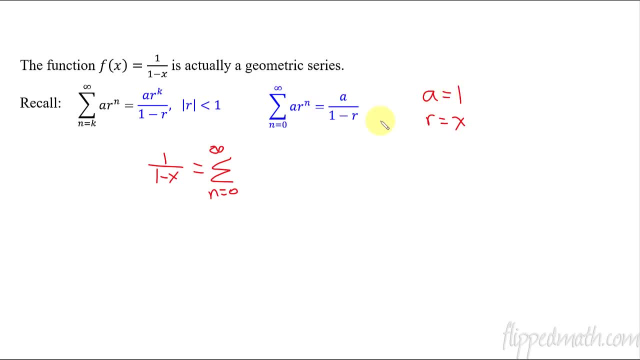 The a is a 1, so I don't have to write that My r is an x, so I'm going to say x to the n. That's what this 1 over 1 minus x equals, Or in other words, it is equivalent to 1 plus x, plus x squared, plus x cubed. 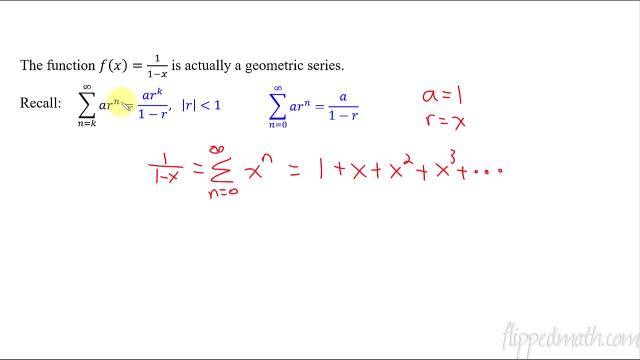 And that's it. It's that easy of a pattern, Okay, kind of a cool thing that fits in with Maclaurin's series, but also that this thing actually represents a geometric series. All right, let's do some examples. 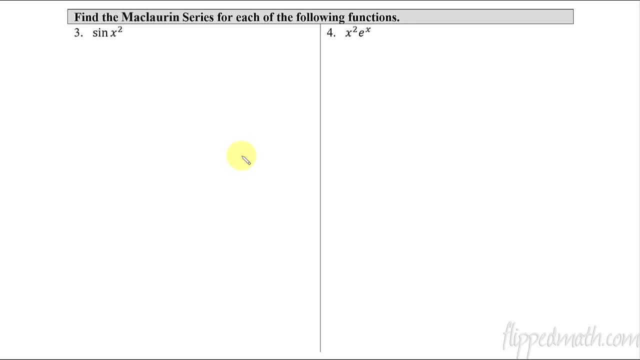 We just got two examples here. so just pay attention real carefully because this is how you're going to do the practice problems. So every time you have one of these, this is how it's going to help you memorize it- You look at what is kind of the parent function of these four. 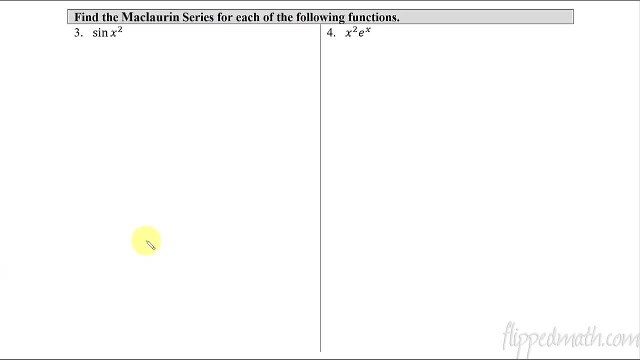 So we're working with one of these four things. Obviously, for this problem it is sine x, So we're going to write down what is sine x equivalent to, And if you write this out, it'll help you to memorize it. 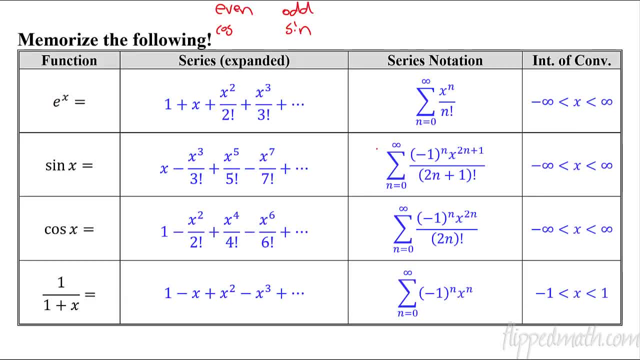 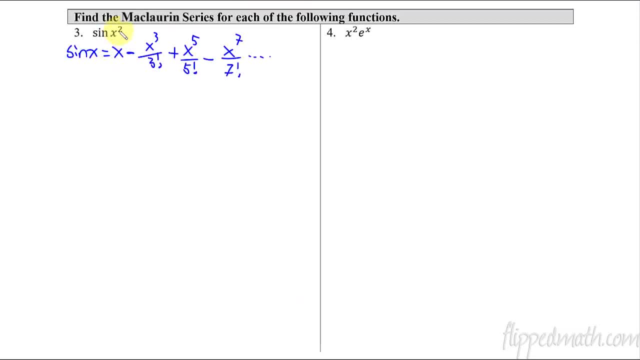 So remember sine And cosine. Sine comes after cosine, So that's going to be the ones with odd. So you've got to go odd, odd, odd, odd. So we're going to write it out again. So what we're doing with this in order to get sine of x squared. 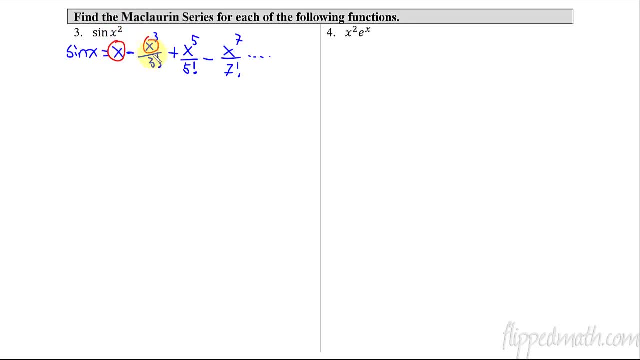 all you have to do is every time an x shows up. so each of these you're going to, instead of x, you're going to put whatever. this is an x squared in this case. So what we can say is that a sine of x squared is going to equal this exact same thing. 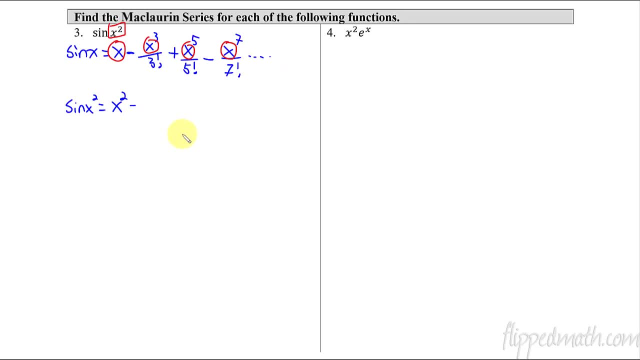 but instead of an x it's x squared. So this is x squared, minus x squared, raised to the third, over three factorial. So this would become x to the sixth if we simplified it, And then plus x squared, raised to the fifth, over five factorial. 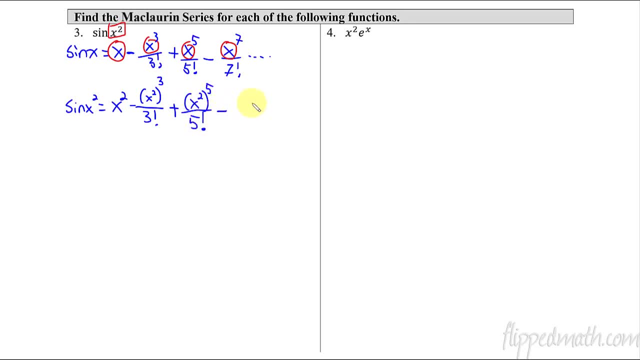 And again this x squared to the fifth, that would become x to the tenth. And then, minus x squared to the seventh, over seven factorial, That becomes x to the fourteenth. And we just keep continuing that pattern over and over and over again. 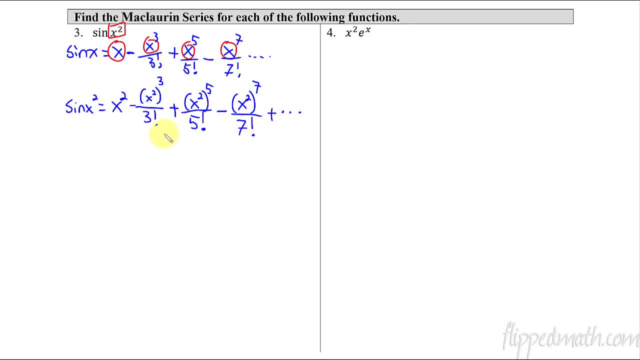 Now, what we needed to figure out as well is, if we had- well, let me say this Many times, the problems will just say what are the first three terms, And so you just write this one, this one, this one, and you're done. 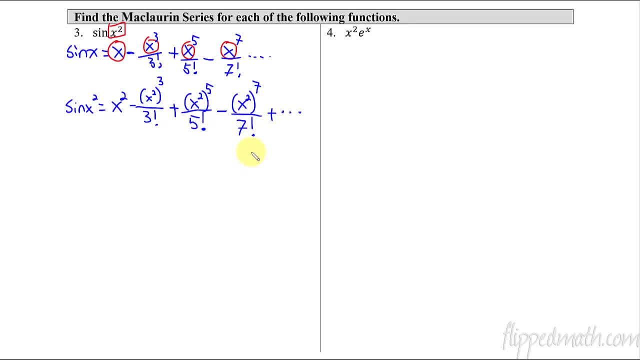 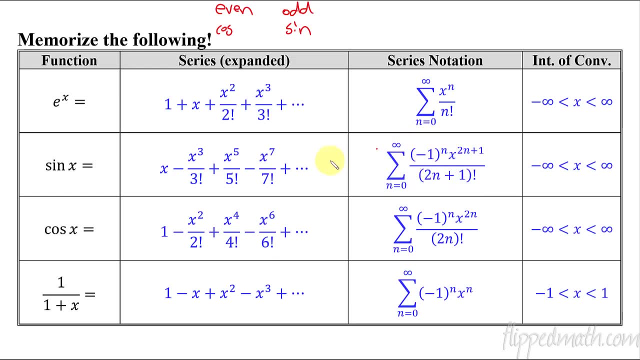 Or maybe the first four terms. So one, two, three, four and then you're finished. But you also might have to figure out the summation notation part, This part, right here. So how does this change? Okay, so I've taken this thing. 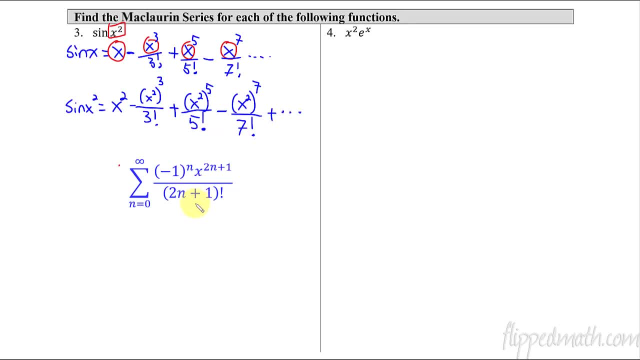 This is sine x, the summation notation for sine x, And let's change it. What are we doing? The x is going to become an x squared, So that x. So what does that mean? We're now going to have from n equals zero to infinity. 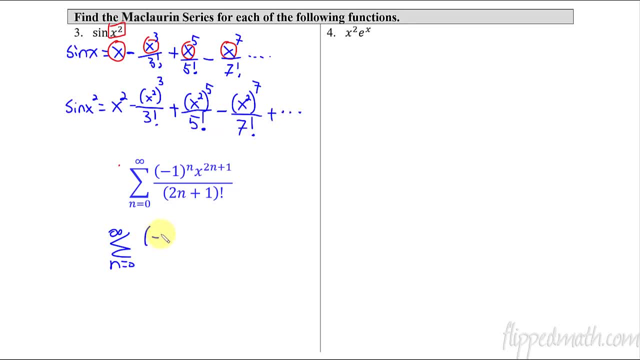 I'm so sloppy with these summation notations. Negative one to the nth power, And now this is x squared to the two n plus one, all over two n plus one factorial, And they might simplify this. So if it was a multiple choice, you might then have to even go one more step. 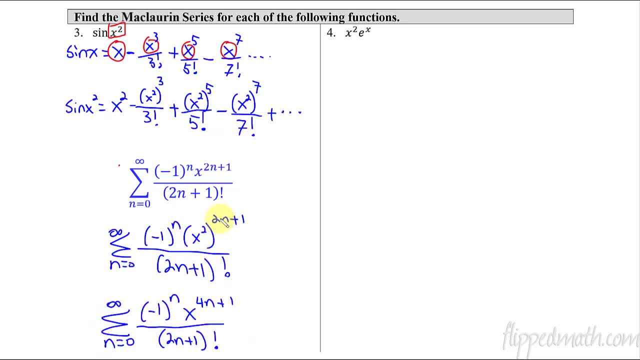 And it comes out and looks like this: Because power to a power, you multiply, So it's two times two n, two times, Oh, what's supposed to be one? Whoops, right there. Okay, fix it. There we go. 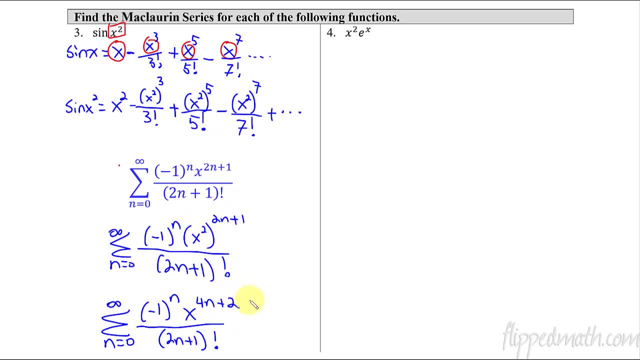 Four, n plus two, So two distributes, because it's power raised to a power and you multiply. All right, So that is this one. So this would be the series written out expanded And then this would be the summation notation here for the series: 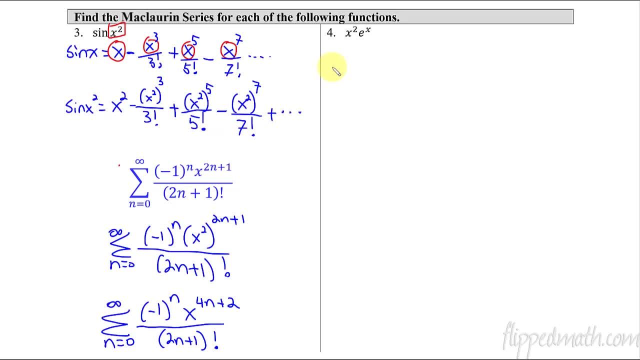 All right, One more problem And then we're finished with this. So e to the x, e to the x. Let's start off. This is how you want to do this, And I would do this on your practice problems, to write out what the original one is before. 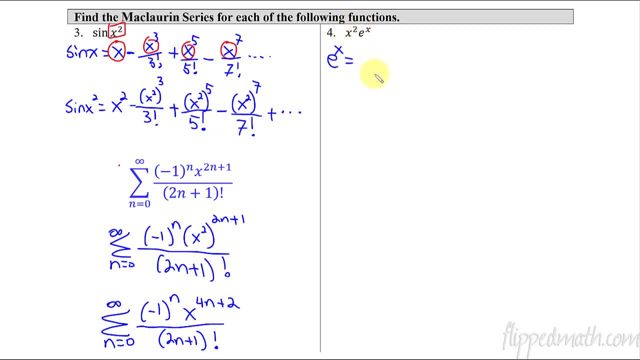 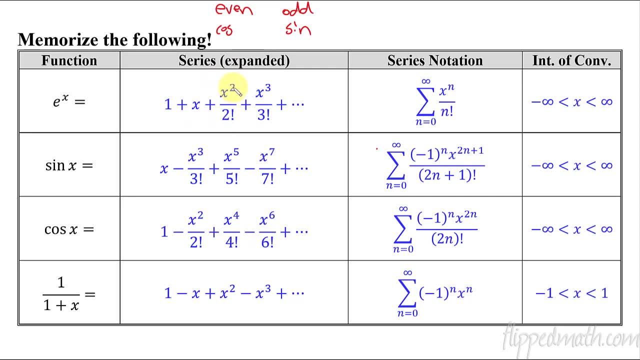 it's been manipulated and modified. So our e to the x. You remember what that is. Can you remember without looking? That's one plus x plus x squared, So it's always just over the exponent factorial three, three, factorial four, four, factorial. 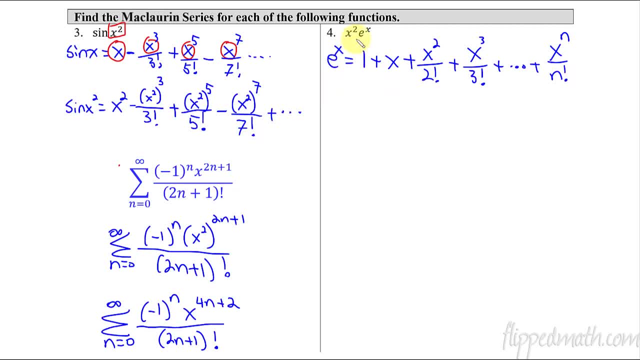 until you get this thing long thing here. All right, Now what do we do next? What is happening is we've got x squared times, e to the x, So you've got this entire series here that's just getting multiplied by x squared. 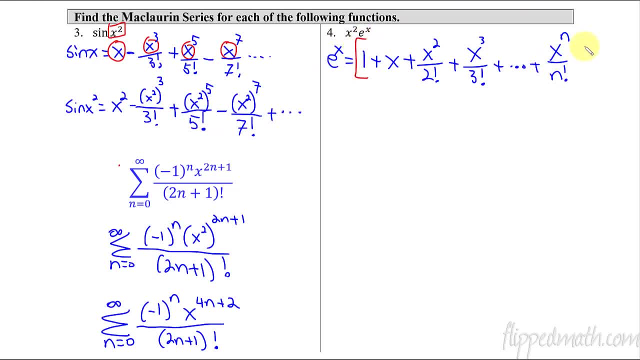 So all we have to do is you take this whole thing and you're going to multiply it by x squared. So what we say is that x squared times e to the x is going to equal. and now each one of these terms, multiply it by x squared. 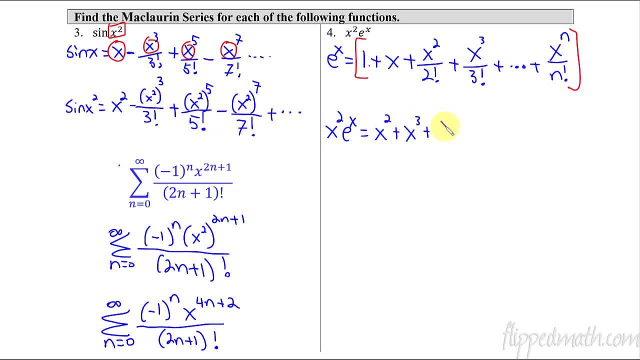 So that's x squared plus x cubed, plus x to the fourth, But now the bottom doesn't change, So it's two still two factorial. or you can just say two plus x to the fifth power, because we're just adding exponents three factorial, and I don't know why. as I'm writing, it's: 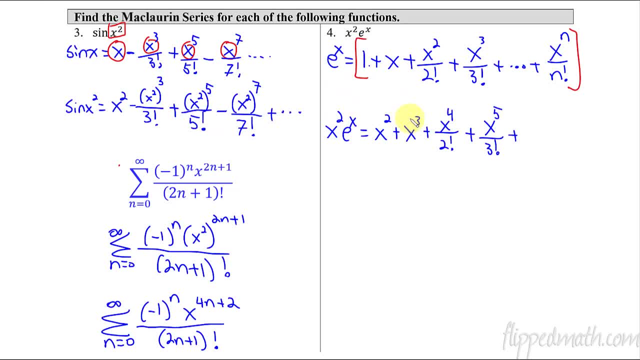 getting bigger. You notice that it's like getting bigger as I go to the right. Sorry, Dot dot dot Until we get to the last term. And how do we do this? So you have to think: what's x squared times x to the nth. 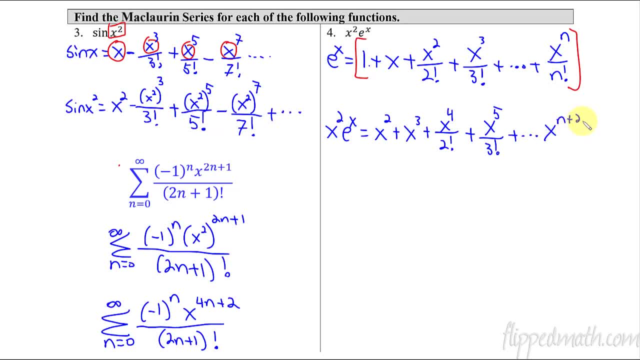 You add exponents, So it's just n plus two inside the exponent all over n factorial. And that helps us out quite a bit, because if you've got that nth term then when you jump to the summation notation you just go from zero to infinity. 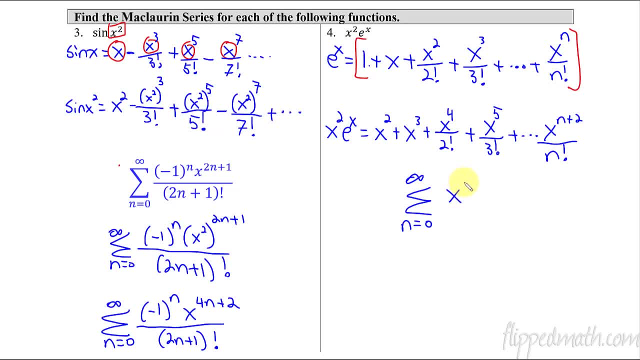 That was an awful infinity. And then that is the nth term. So we're summing up all of the terms that are from zero to infinity of this thing. All right, And then that would be your answer. Well, both of these are your answer.